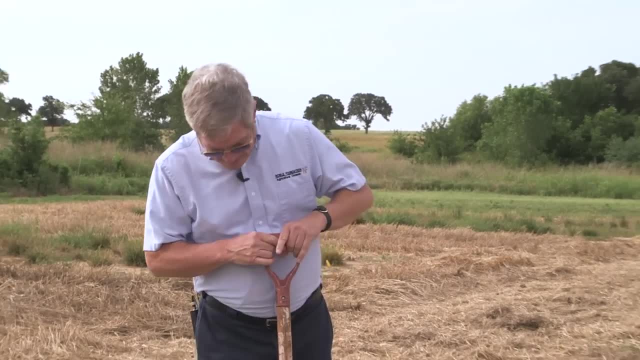 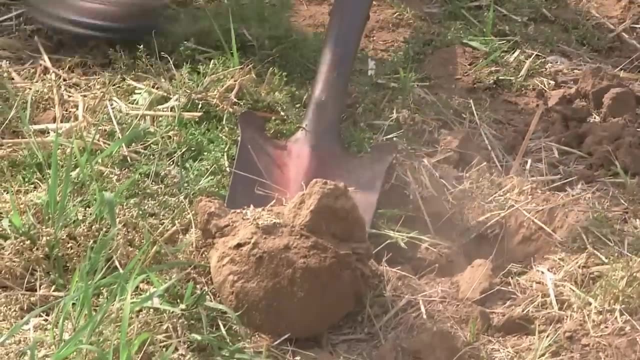 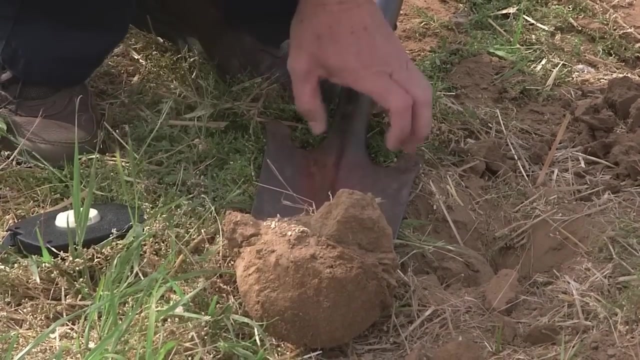 you could use a shovel instead, and the way you do that is: you go down, you dig a little deeper than 6 inches, bring the soil up. Now we only need 6 inches of this soil, so if I take 6 inches from the top, it comes to right there. I then need some tool to stop. 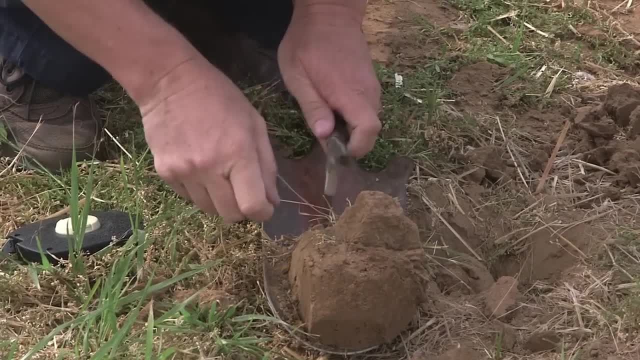 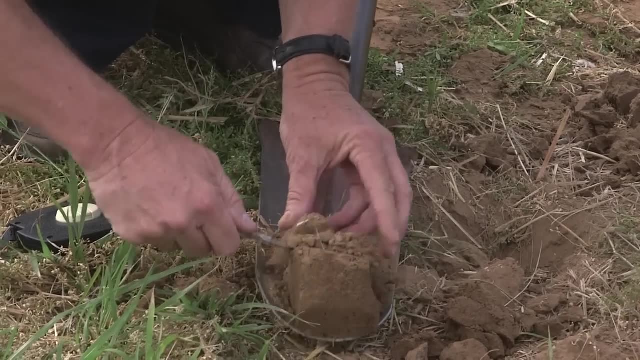 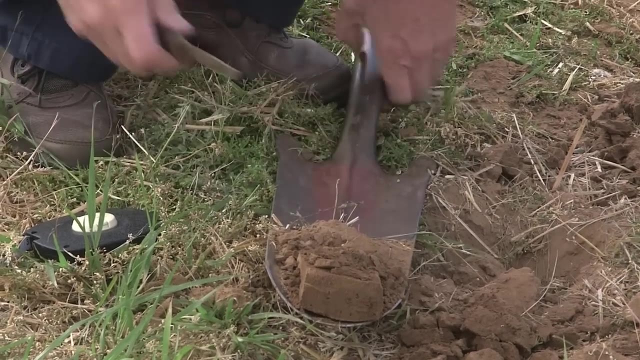 it at 6 inches. Get rid of the rest. Then we need this to be kind of uniform. We want a core, a sliver of this instead of the entire amount. So here now we have a 6 inch sample, We put it into. 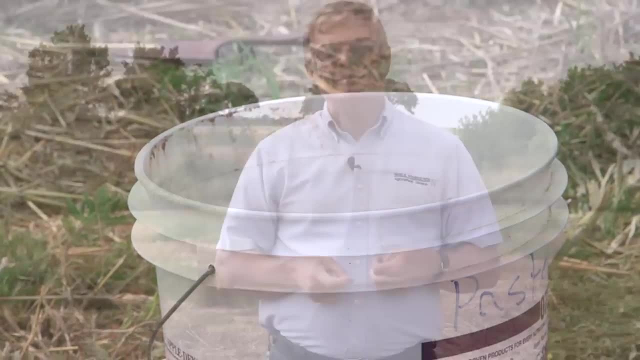 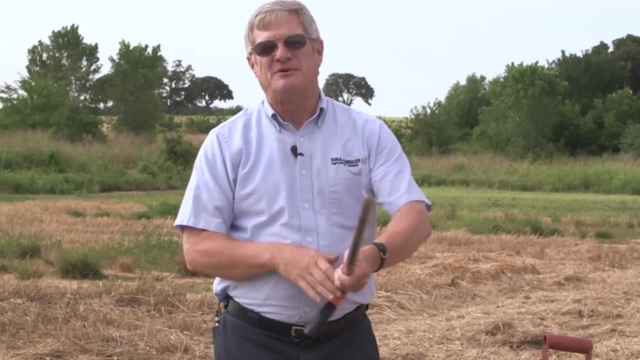 the bucket. That's a fair amount of work. If you're going to take very many soil samples in your life, you would be well off to either buy or borrow a specialized soil sampling probe. Now, a soil sampling probe is not good for anything except taking soil samples. So if 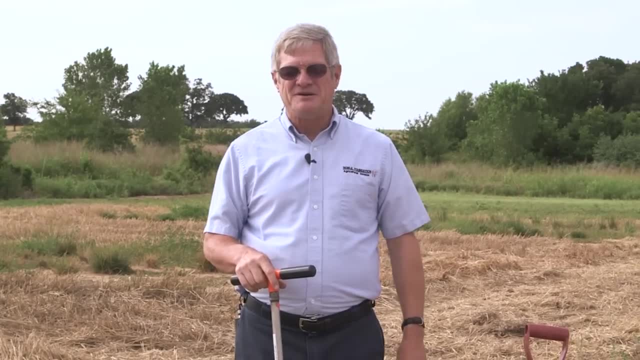 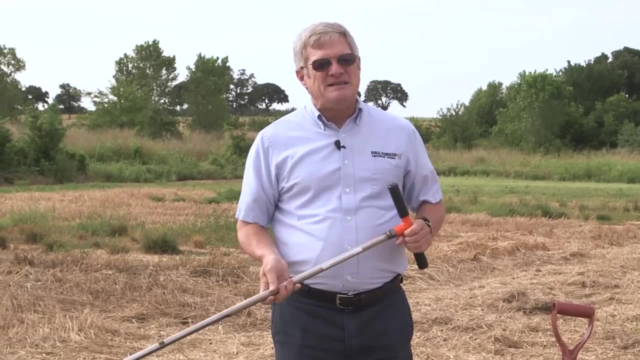 you don't plan to take but 3 in your life, it's not worth buying $50 to $100 for one of these. However, if you plan to take many, then this will be a great thing. Sampling depth is critical. You may have noticed I used 6 inches on the last one, The sample. 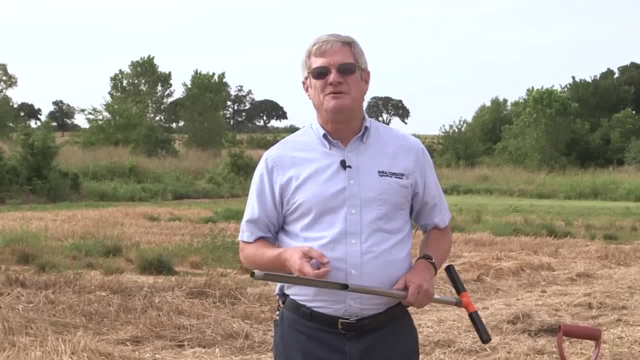 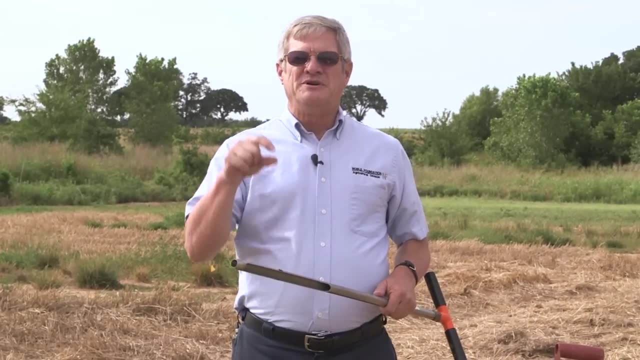 has to be taken at a depth of 6 inches for general nutrient analysis. The reason for that is that the nutrients are stratified. The nutrients are stratified and they're not stratified in the soil. There are more nutrients in the upper part of the soil than 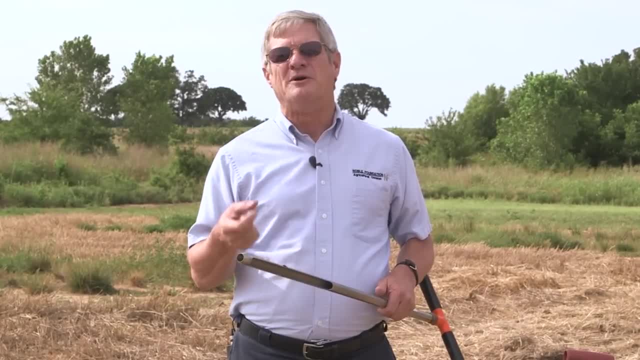 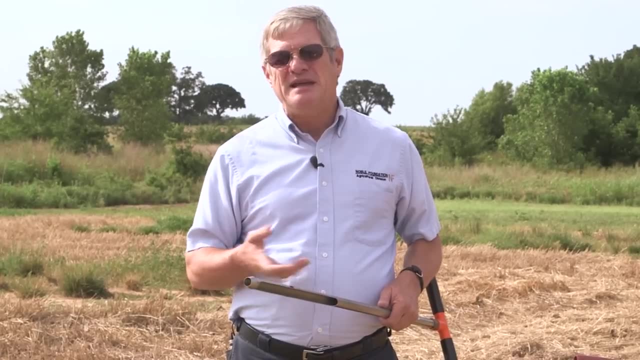 they are in the lower part of the soil. So if you take a sample shallower than 6 inches, it'll look like you have a better amount of nutrients than you actually do. If you take the sample deeper than 6 inches, it will look like you have fewer nutrients than you actually. 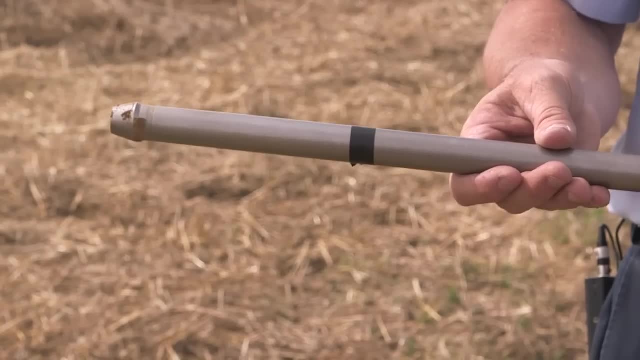 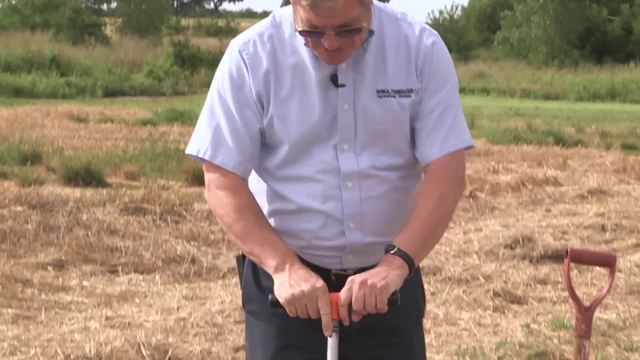 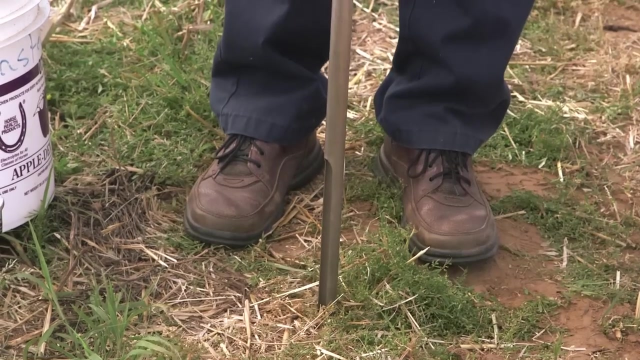 do. You may notice that I've made a 6 inch mark with some electrical tape on my sampling probe so that I don't have to guess where it is. So with this you just push it down, put it down into the ground to your 6 inch mark, give it a quarter, turn The quarter. 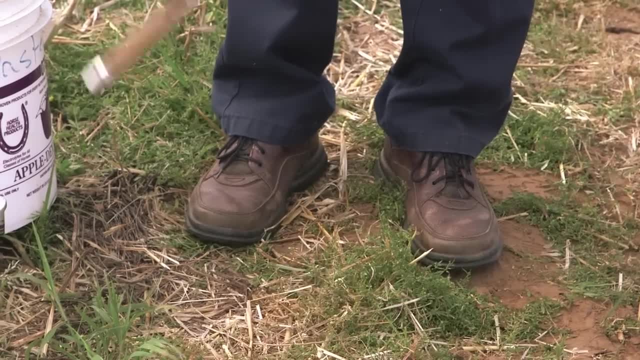 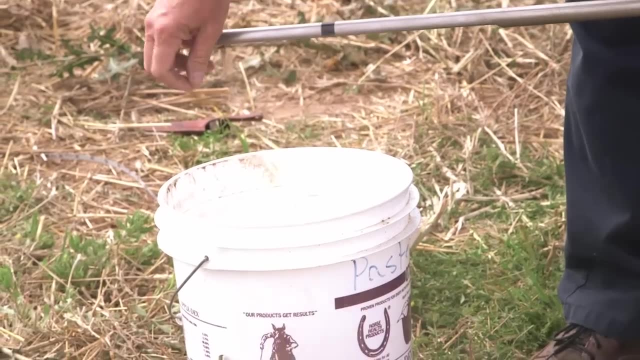 turn keeps the soil in the probe. when you remove it, You bring it out. You've got a nice 6 inch core of soil there. Just put it into your bucket. Whichever way you use, you have to repeat this 10-15 times through the field to get. 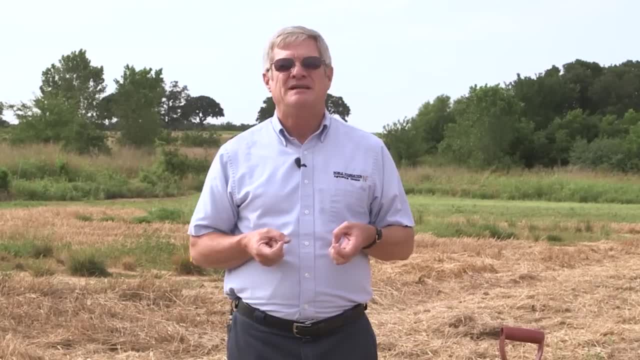 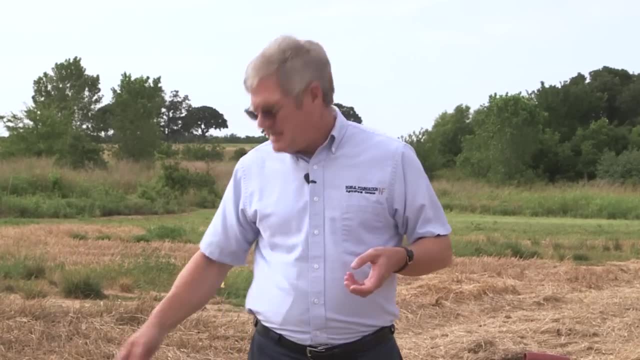 one sample. What I just did is not a sample. That's called a core or a sub-sample And you need 10-15 times 10-15 cores or sub-samples to make up one sample Once you have gotten your 10-15 cores. 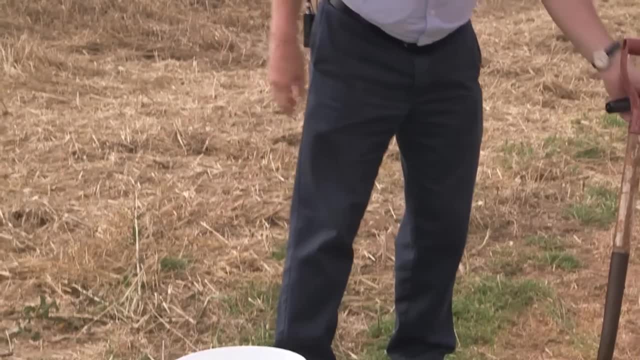 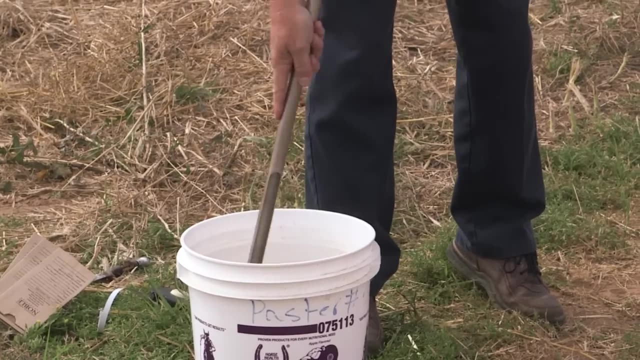 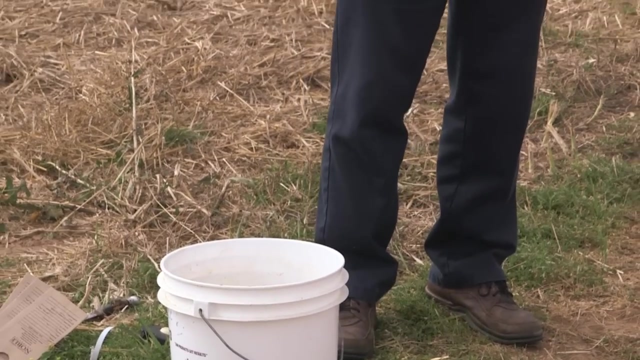 and you have soil in your bucket, then you thoroughly mix it with either your soil probe or a stick or whatever you wish. You mix it up good And unless you like paying a lot of money for postage, you don't want to mail all of. 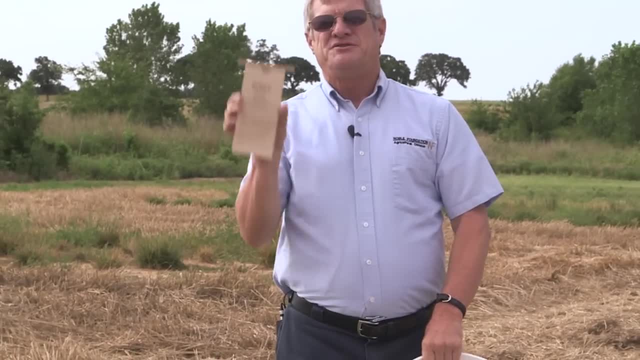 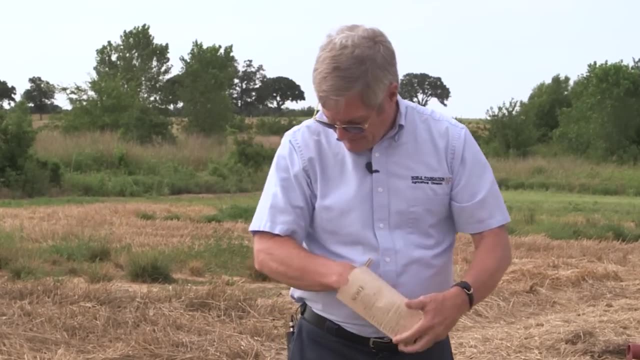 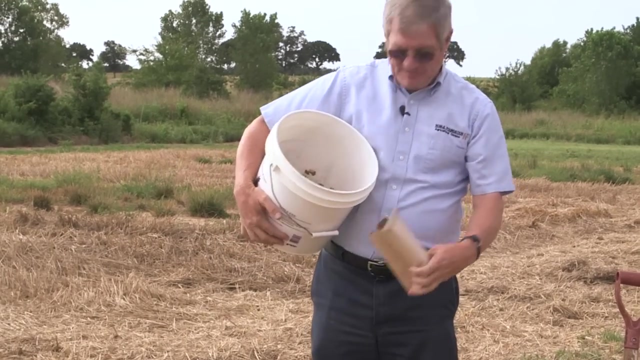 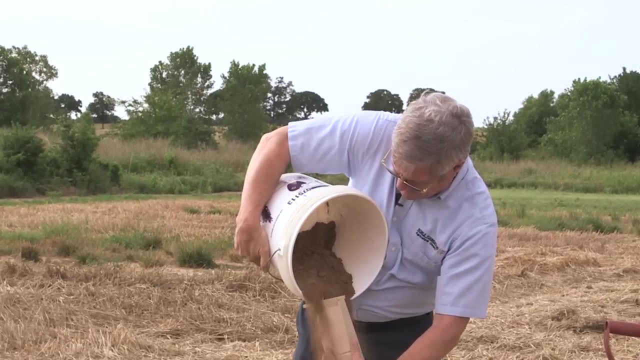 this. We need about a pint in the lab. So you use a container that will hold about a pint of soil and you pour. Since it's all mixed up, it doesn't matter if you spill some. Then you put about a pint of soil into this bag and I have gotten about a half a pint on my arm. 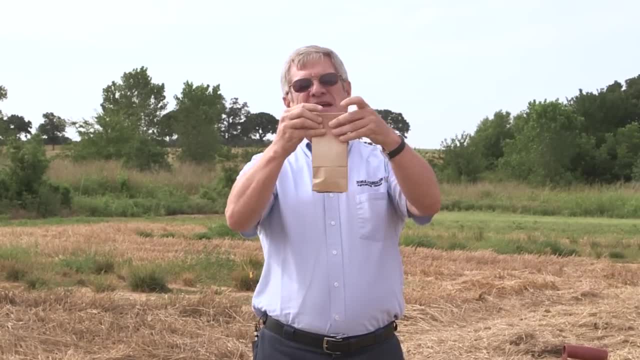 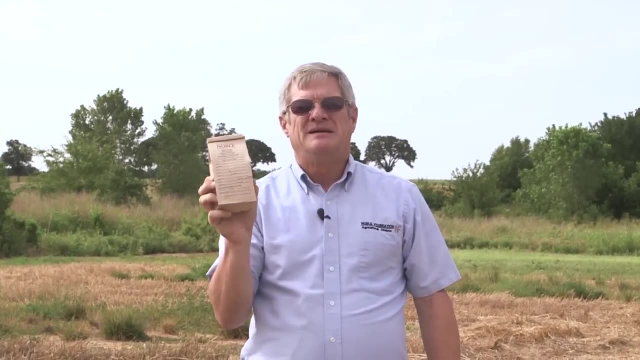 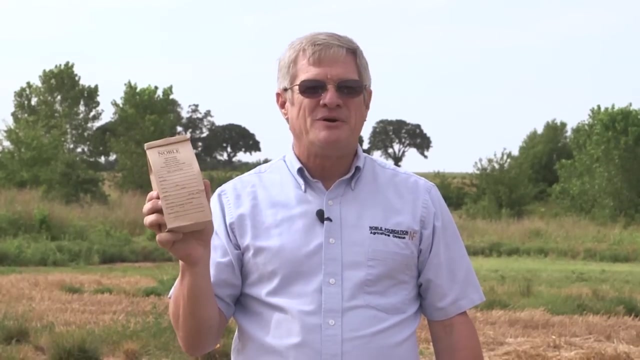 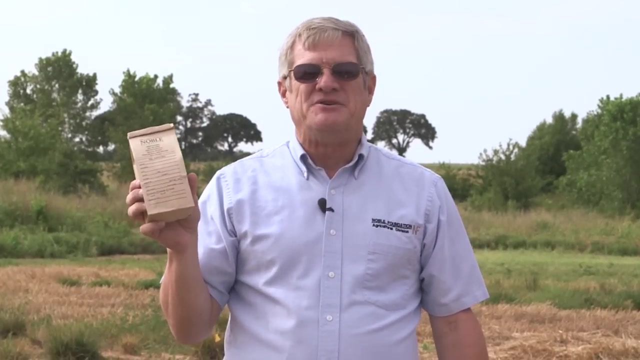 so this is your sub, this is your sample. once you get your sample, we need some basic information on the, the container that you put the sample in. we need, at a minimum, your name, address, phone number, what the name, what the ID of the sample is and what crop you're growing. obviously, we need your name or we don't. 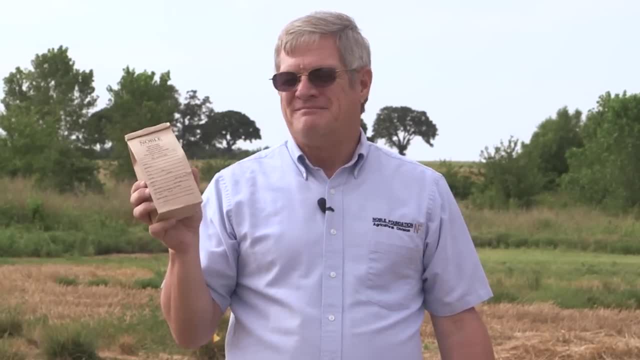 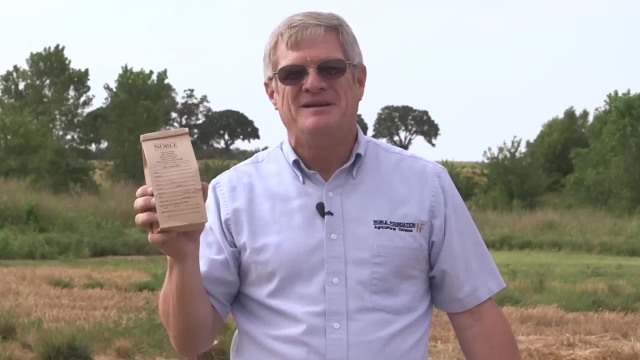 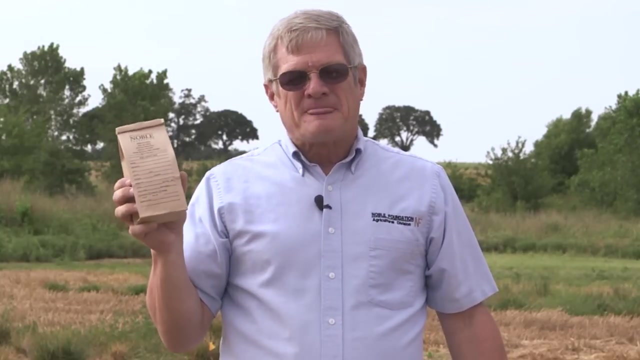 know who you are. we get quite a few samples in our place that don't even have a name on them and basically we just throw them out because there's nothing we can do with it. then we need your address so we know where to mail your, your results to, or your email address at a minimum. then we need to. 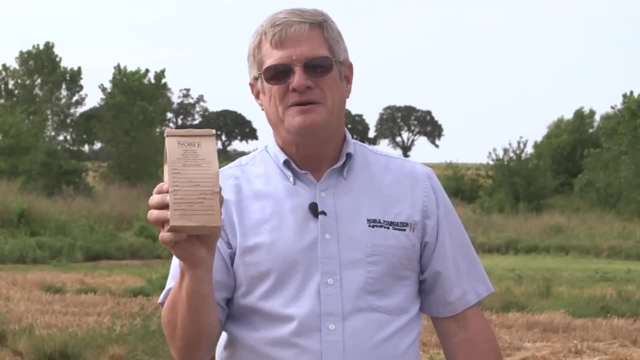 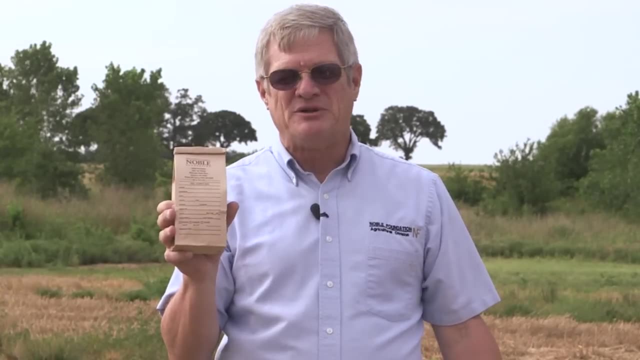 know, or you need to know, what this sample is called. if you send in more than one sample, you have to differentiate them some way, or else you're not going to know which sample is which. if they have different fertilizer and lime recommendations, then we need to know what crop. 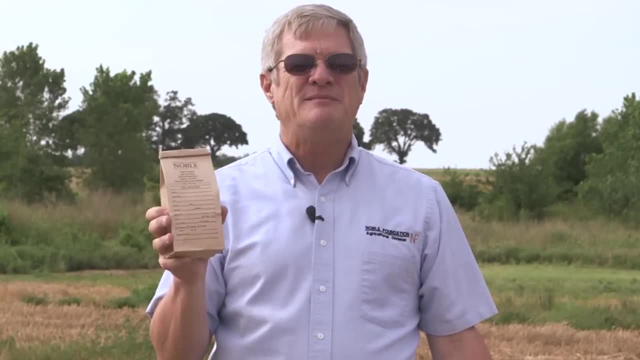 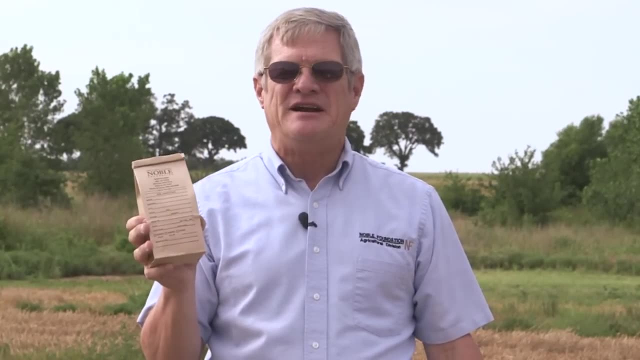 you're growing so that we can make fertilizer recommendations. can't really make a fertilizer recommendation on an unknown crop they've. our recommendations are very specific to a crop and vary depending on which crop you are growing and also what yield goal you have. so if you're after a particularly high yield, 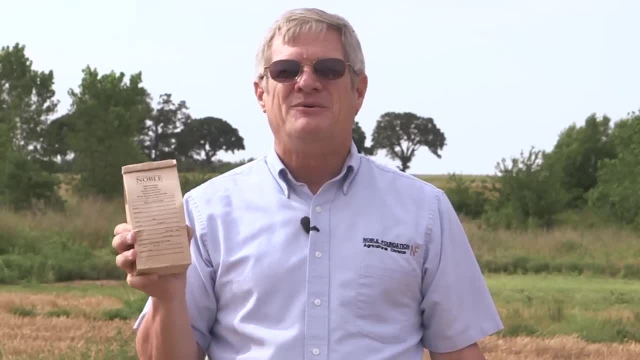 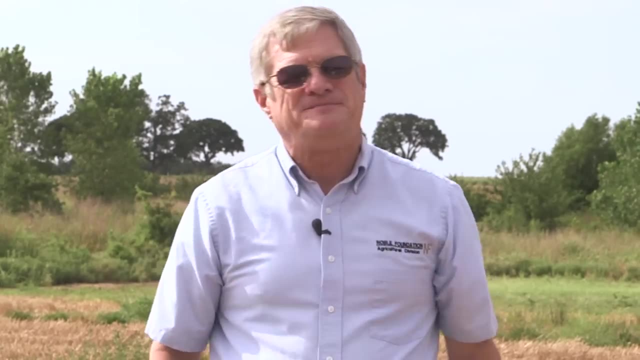 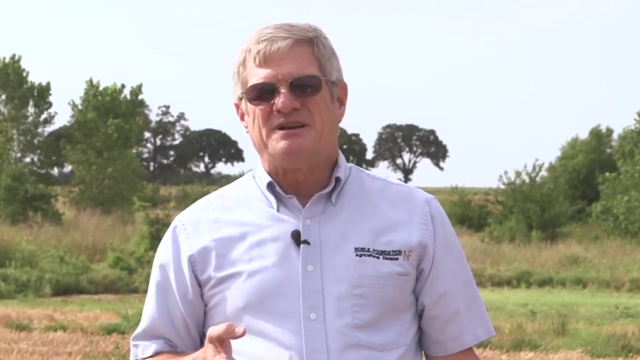 goal, or if you're a particularly low input person, we need to know that. so in order to make a good fertilizer recommendation now, then let's say that you have a field that has a lot of odd spots in it, or even one odd spot in it. say, there's an area in 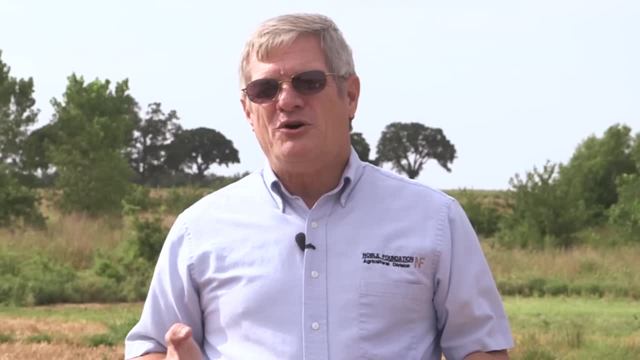 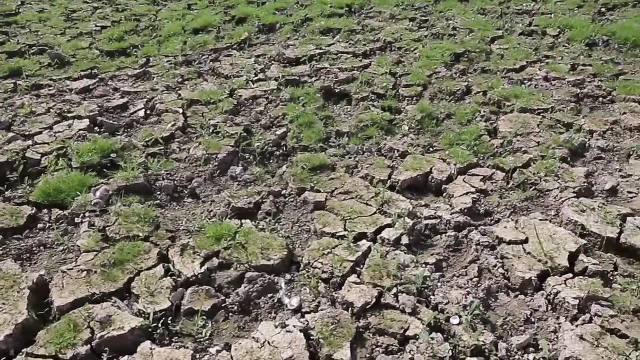 this field that doesn't grow anything. you don't want to include that area in your sample. if you do, it'll just make the rest of your sample look a little bit worse and you won't know why the bad area is bad. so sample that bad area. 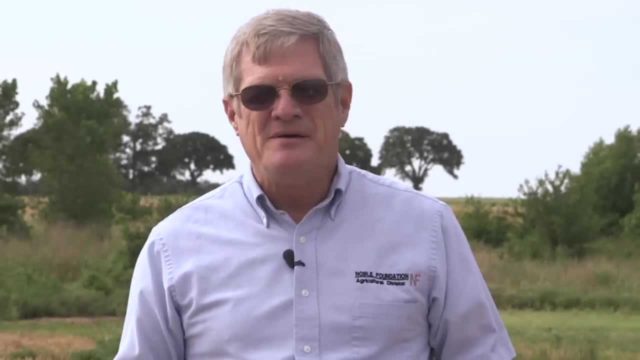 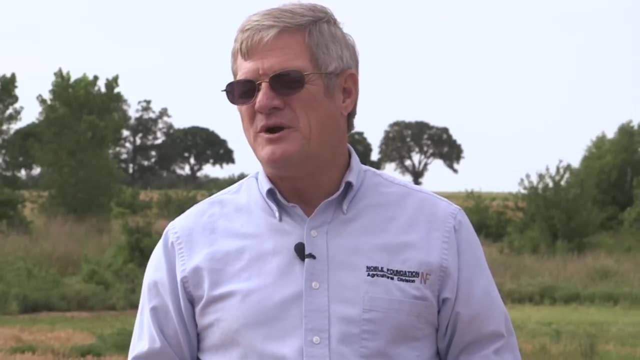 separately and the way you do it. if it's just an acre, you go out and you take soil from 10 to 15 places at random, just like you would in a regular sample. if it's an area where you feed hay in the winter, you would feed. you would do that separately because 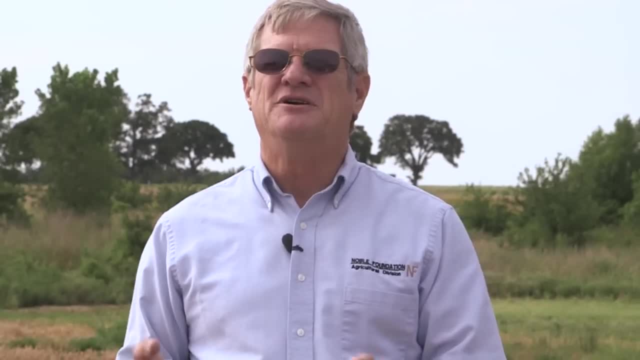 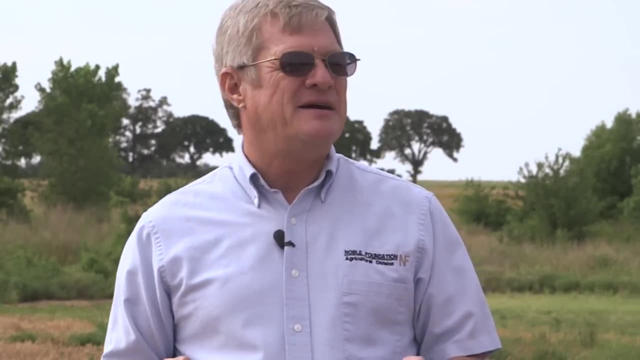 it's likely to be much higher in nutrients than the others, and if you include it, it's going to make the rest of your sample look much better than it actually is. so problem areas or odd areas: sample those separately. when do you want to do this? it really doesn't make a lot of difference as long as you do it at the same time each year. your soil pH and phosphorus and potassium levels can vary fairly greatly depending on what time of the year you're doing it. so if you begin your sampling in the spring, try to sample in the spring every year. if you begin your samplings in the fall, try to sample in. the fall every year. that way, you will have a consistent background on which to compare your your soil from year to year. how often do you need to sample generally, if you're looking at just phosphorus and potassium and pH, probably every three years is enough, unless it's a very unusual case. 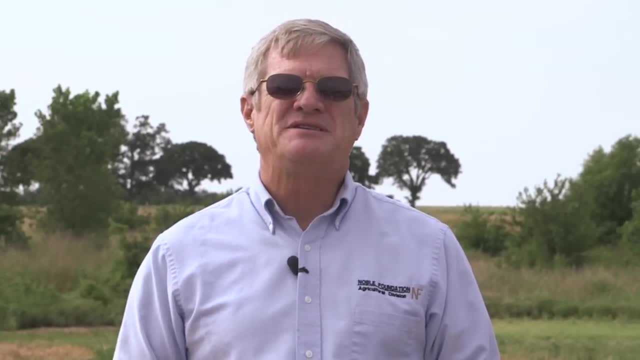 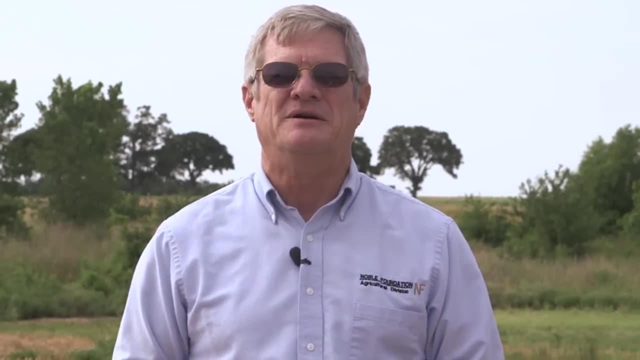 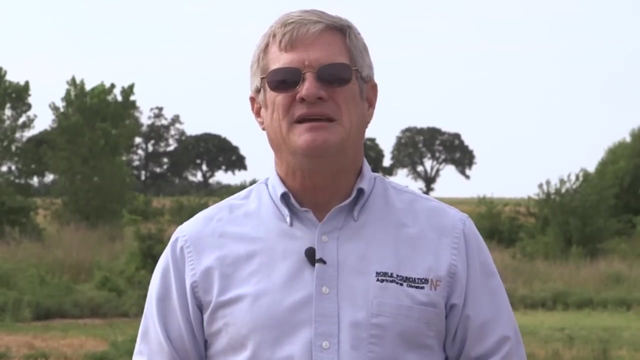 however, if you're looking at nitrate nitrogen, then you need to sample that, probably within 30 days of when you're going to apply the fertilizer, and then that analysis is only good for that year. nitrogen is very dynamic. in the soil it changes forms, it's taken up by the plant and used it can be lost in heavy. 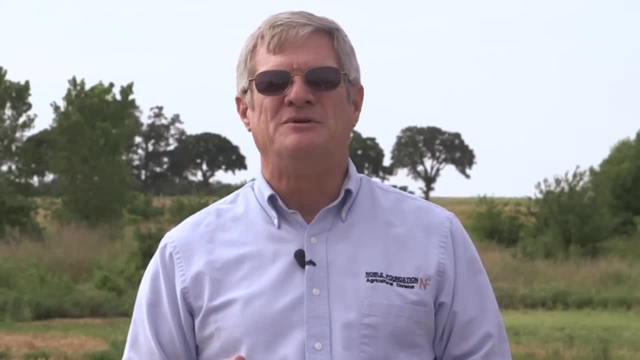 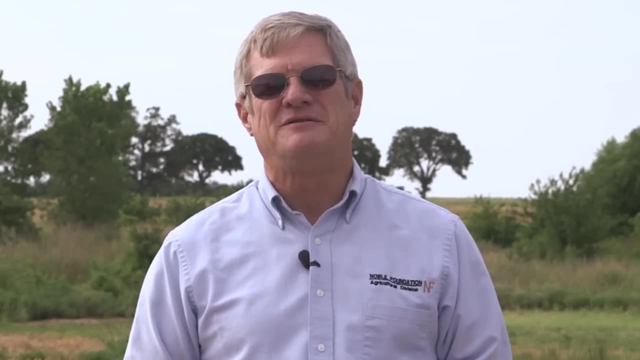 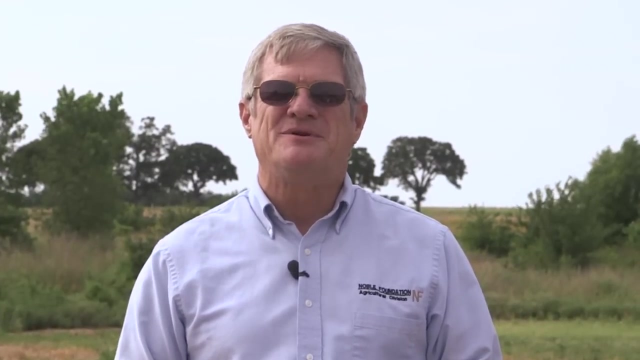 rainfall. so nitrate nitrogen analysis are only good for a couple of months. pH, P and K recommend analysis are probably good for several years. so basically, based on that, a good soil sample can give you a basis on accurate fertilization. however, you need to take the sample correctly: taking the sample. correctly involves sampling to a six inch depth, no more or no less, taking 10 to 15 cores within that field, stirring those up good and taking a pint of that as your sample. so, with that said, good luck on your soil testing program you.